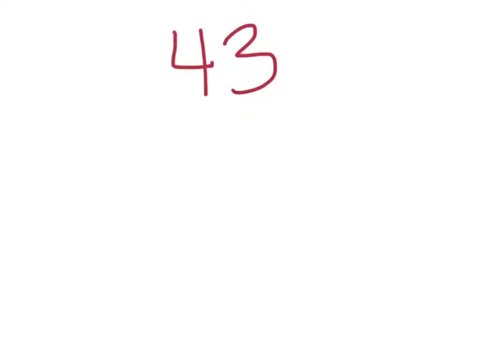 And I'm going to show you how to do that. So what happens if your book gives you the number 43? Well, what you're going to do is you are going to reverse the digits, So you're going to bring the 3.. 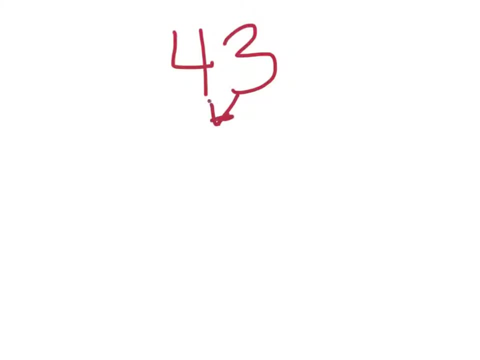 You're going to bring the 3 into the 4's place, which would be the 10's place right, And the 4 into the 1's place and make it 34.. Then on your calculator. yes, you may have calculators today, woohoo. 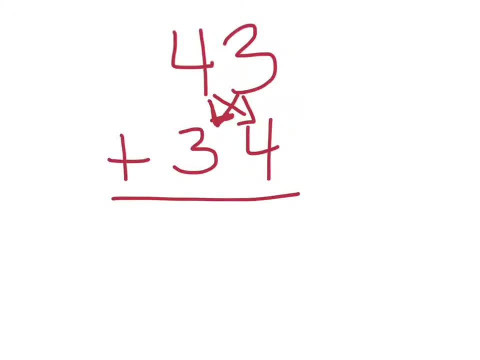 you are going to add those together. When you add those together in your calculator, you will get the number 77, which you will notice is a palindrome. From this direction it's 7-7, and from this direction it's 7-7.. 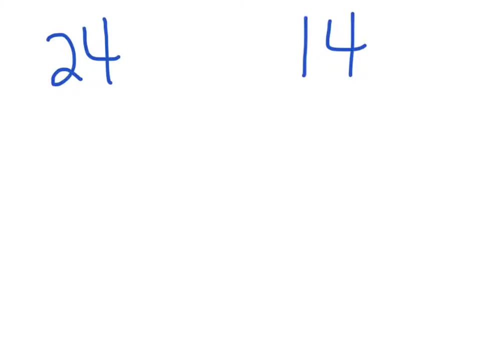 Here are two more numbers that we can turn into palindromes. So here's: the first number is 24.. So we are going to again reverse the numbers and add them together. So instead of 24, I wrote 42.. 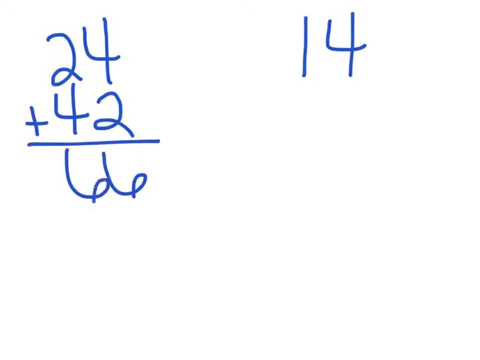 And if we add them together in our calculators we will get 66. So this is a palindrome: 66 from this side and 66. Now 14,. we would reverse the numbers, put the 4 in the 10's place and the 1 in the 1's place. 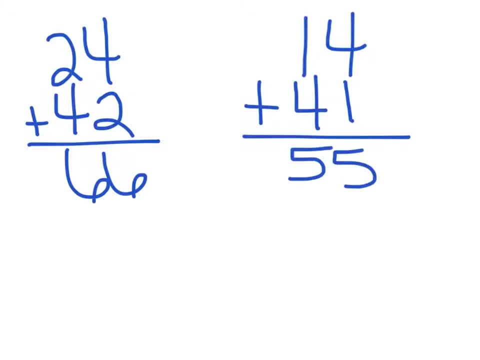 Add them together, we get 55.. Again, we've created a palindrome. Sometimes, in your calculations, though, you will run across a number that needs more than one number added to it, For instance 73,. if you reverse the numbers, you get 37.. 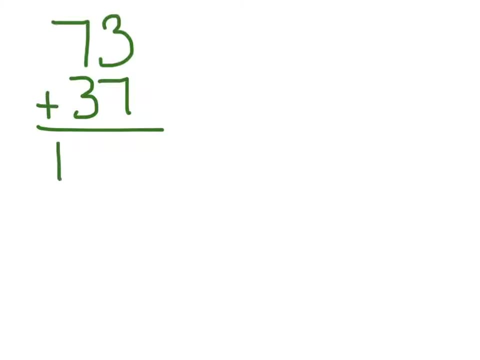 If you add those together in your calculator, you will get 110.. 110 is not a palindrome. From this side it's 110, and from this direction it's 011,, which is not the same. So we need to add another reversal.